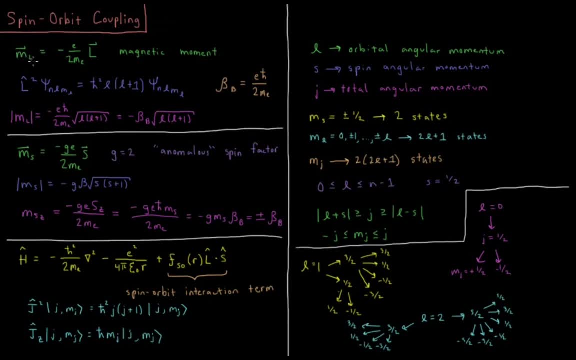 So our magnetic dipole, based off of our orbital angular momentum, of the electron in its atomic orbital, We have the angular momentum squared operator, or shall I say orbital angular momentum squared, L squared acting on psi, nL, m sub L, m sub L is now noted because we're going to have spin angular momentum as well. 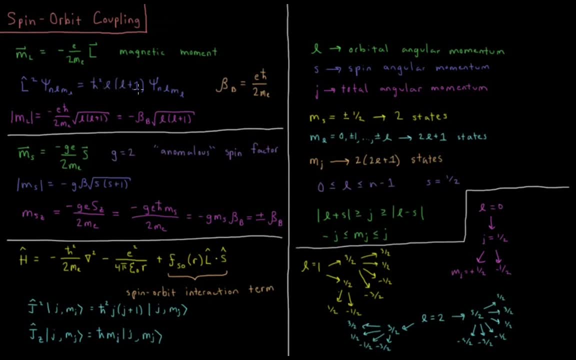 That equals h bar squared L times L plus 1 times psi, nL m sub L. So psi is atomic orbitals, or eigenfunctions of L squared with an eigenvalue of h, And we have the absolute value of this angular momentum vector is thus going to be the square root of that. 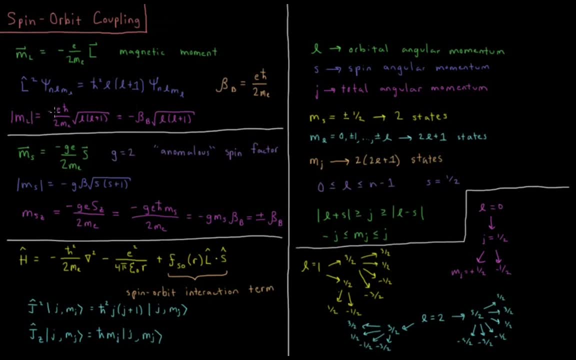 So our magnetic moment from this is going to be minus e h bar, over 2 times mass of the electron times, the square root of L times L plus 1.. Note that from the Zeeman effect video, the Bohr magneton beta b. 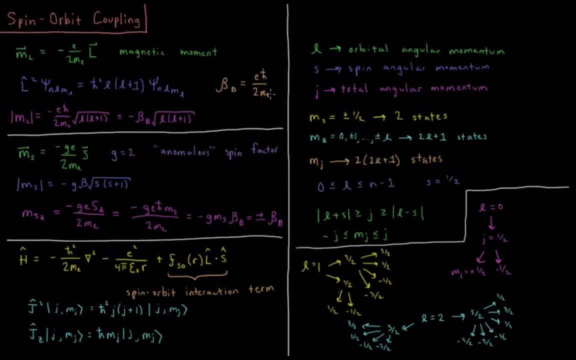 equals e h bar over 2 times mass of the electron. So our magnetic dipole moment from angular orbital angular momentum is going to be negative Bohr magneton times L times L plus 1.. All right, so that's the magnitude of it. 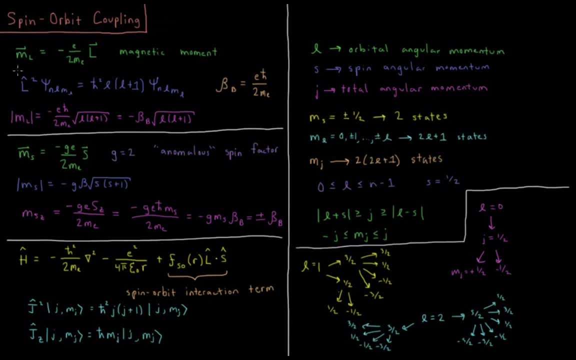 What about for our spin angular momentum? So this is from orbital angular momentum. You can imagine that as the particle rotating around, So that's the magnitude of it. You can imagine that as the particle rotating around the z-axis, But the spin angular momentum, you can imagine that like the particle rotating around itself. 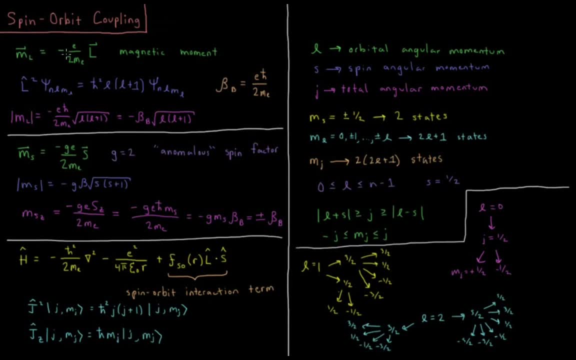 So orbital angular momentum is like the earth going around the sun. Spin angular momentum is like the earth spinning around its axis. So we have to account for the fact that not only is it spinning around an axis, but it's spinning around itself as well. 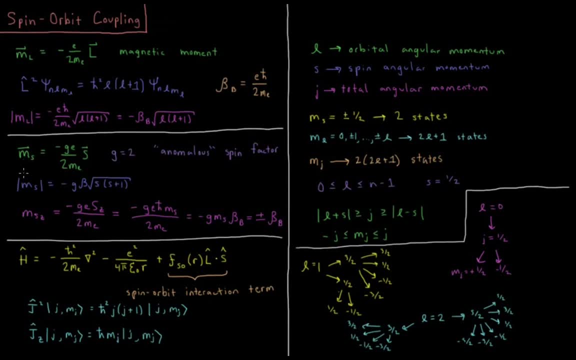 Electron spin doesn't exactly work that way, but that's the analogy that we can use to think about it. So we would get a magnetic dipole moment vector from the spin angular momentum as well, And that's equal to negative g times the charge of the electron, over 2 times mass of the electron times, the spin angular momentum vector. 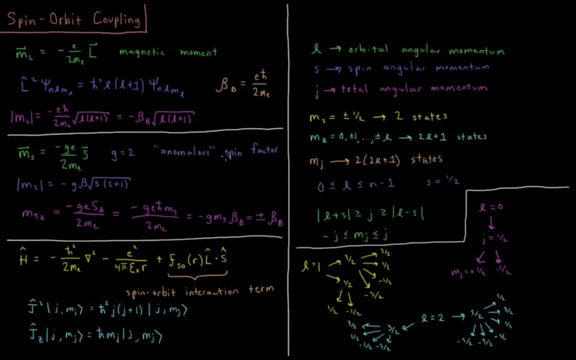 This factor g is just equal to 2.. That's called the anomalous spin factor. You for some reason get an extra factor of 2 in this magnetic dipole moment relative to this one. So similarly we have. it is an eigenfunction of the s-squared operator. 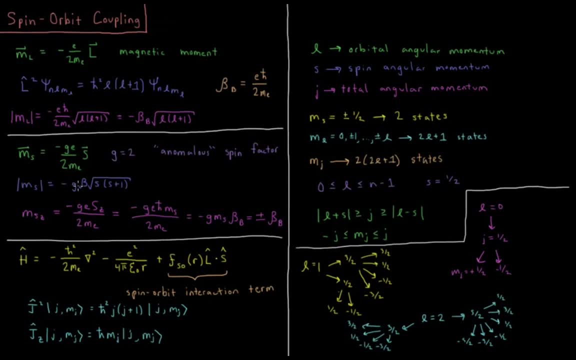 So absolute magnitude of m sub s is negative. g, bore, magneton, beta times, s, times s plus 1.. s for an electron is 1 half. Remember: the value of l for an electron in an orbital is an integer going from 0 to n for a given principal quantum number. 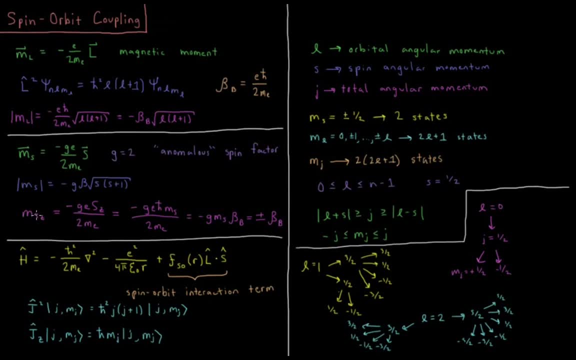 So the z component of this orbital of the spinning your momentum is equal to negative g charge of the electron s sub z times 2 times over 2 times mass of the electron z component of the spinning your momentum, Which is just h bar times m sub s, which we saw from the previous video on electron spin. 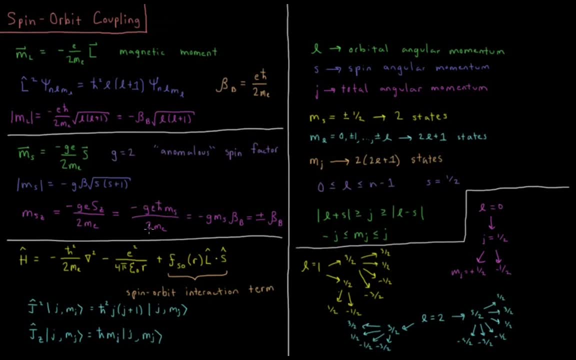 negative g, e, h bar m sub s over 2 times mass of the electron. This is equal to negative g times m sub s times beta b, or equal to equal to plus or minus beta b. g is 2 m sub s is plus or minus 1 half. so we get plus or minus beta b for the z component of our spin angular momentum. 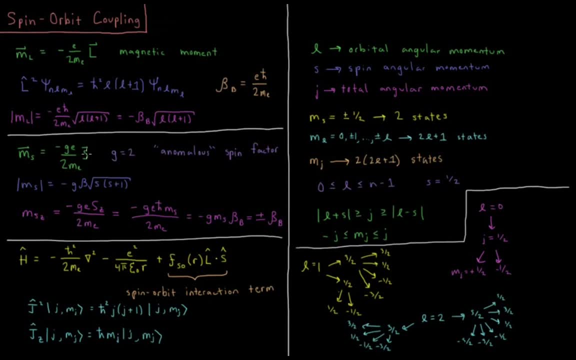 Alright, so we got these two angular momentum on angular momentum going on here. How does this affect our Hamiltonian If we have some kind of magnetic field? So we have. our Hamiltonian is equal to kinetic energy operator minus h bar squared over 2 times mass of electron del squared, the Laplacian operator. 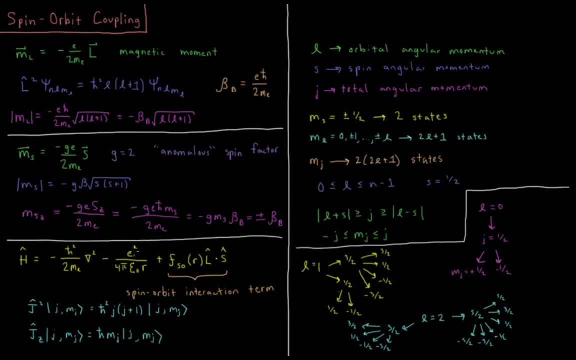 Potential energy from the Coulomb potential minus e squared over 4 pi. epsilon naught r, distance of the electron from the proton, And then we add plus a spin orbit interaction term. So we have our angular momentum from our orbital angular momentum from up here. 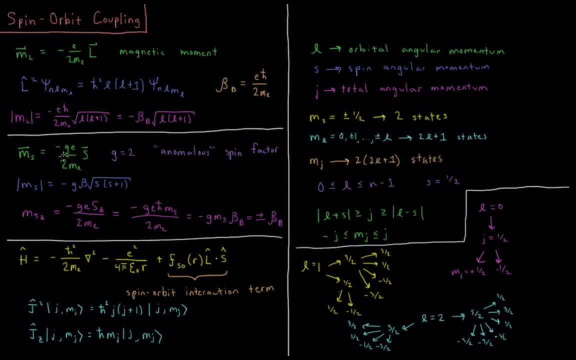 We have our angular momentum from the spin, angular momentum down here, So orbiting around the axis and spinning around itself, And this is some unspecified term which we're not going to mess with further. Basically, this whole video, to this point, the whole point of it, is discussing what we need to do to discuss the quantum number j. 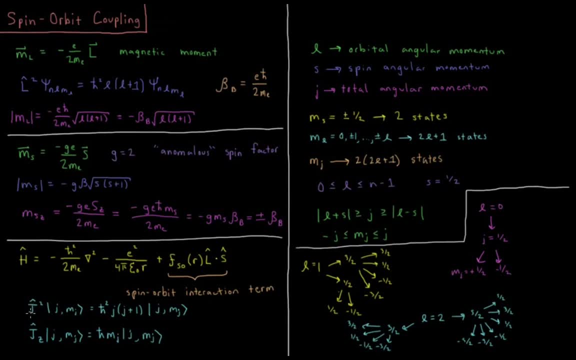 So this is the quantum number j. So j represents the total angular momentum. L squared is the orbital angular momentum. squared S is the spin angular momentum. squared J is the total angular momentum, once we have accounted for orbit and spin. So the operator j squared acting on a state, j, m, sub j. 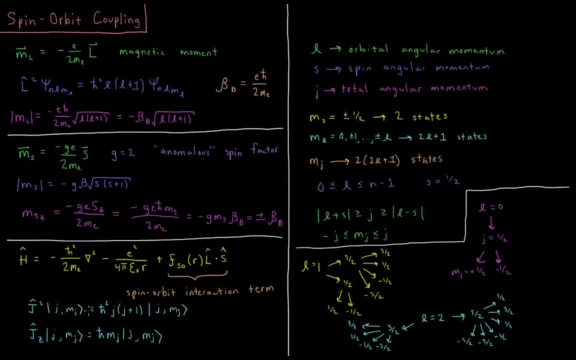 Just like the s squared operator, just like the l squared operator is going to be h bar squared j times j plus 1x. J squared j times j plus 1, acting on that same state, And it also has a z component. j sub z is j m sub j acting on j m sub j equals h bar m sub j, j m sub j, just like l sub z, just like l sub s. 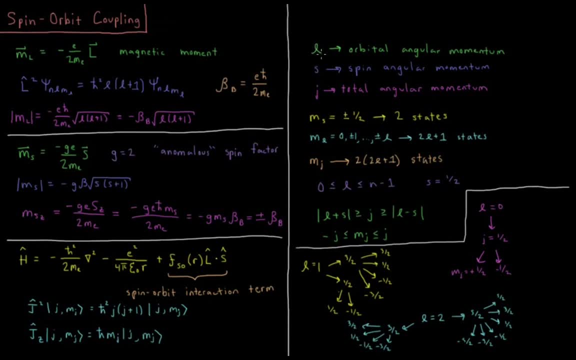 So these three angular momenta, to summarize: L is the orbital angular momentum, S is the spin angular momentum. Those two combine to give the total angular momentum. m sub s, for an electron is plus or minus one, half, Two possible states: m sub l equals 0, plus or minus 1, plus or minus 2, etc. all the way up to plus or minus l. 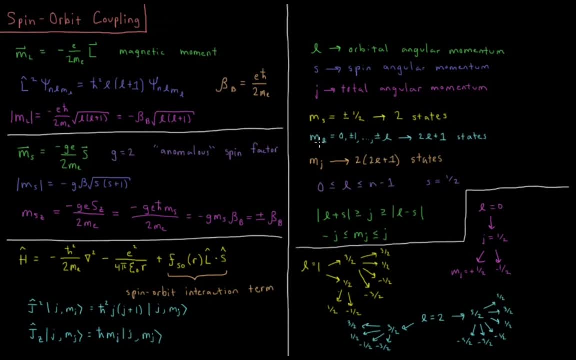 That gives 2l plus 1 states for a given value of l m sub j is going to give 2 times 2l plus 1 states, The two spin angular momentum, The two spin states and the 2l plus 1 orbit states combined to give the product of the result. 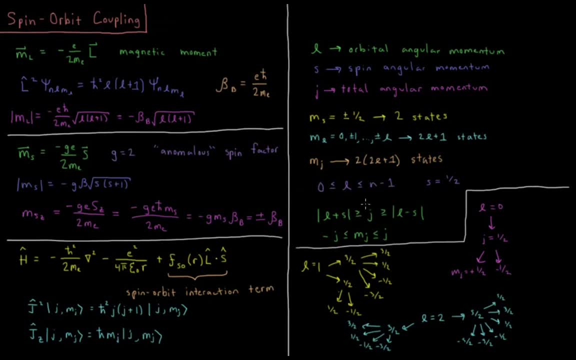 Alright. so what values of j can we have for given values of s and l? Well, j is every integer or half integer going from the absolute value of l plus s down to the absolute value of l minus s, And then m sub j is an integer going from minus j up to j. 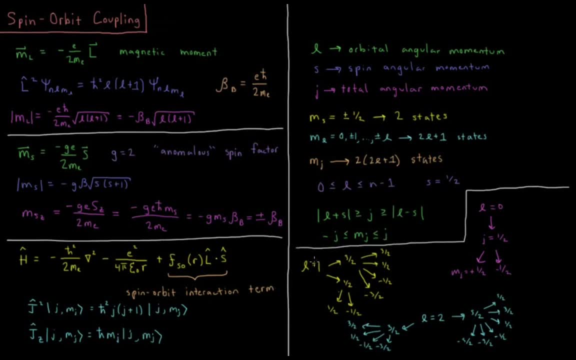 So we'll do some examples here. So if l equals 0, an s orbital we're going to have. j equals one half, because s is one half. 0 plus one half, 0 minus one half is both one half in absolute magnitude. 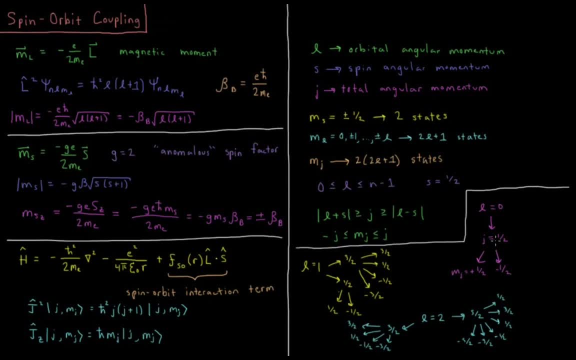 So m sub j is going to equal plus or minus one half for an electron in an s orbital. For an electron in a p orbital, l equals 1.. And j is going to be three halves and one half: l plus one half. sorry, 1 plus one half, 1 minus one half. 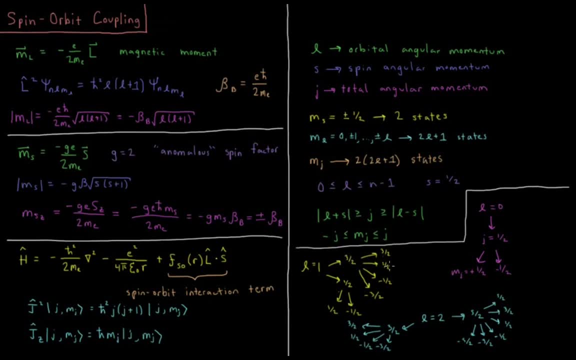 The values of m sub j, there will be four values for three halves, Three halves to minus three halves. For one half it's plus and minus one half. So notice, for l equals 1, there's 2l plus 1 or 3 states. 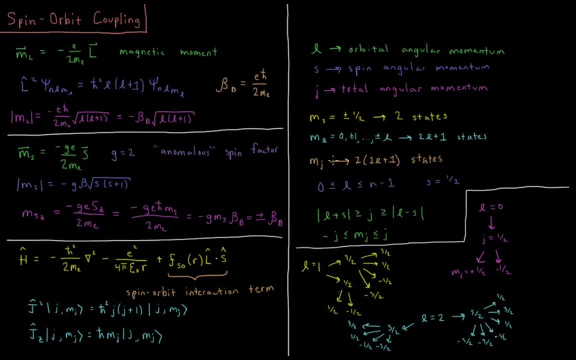 For m sub l, 1, 0, and minus 1.. For m sub j, there's 2 times 2l plus 1, or 6 total states, Even though the plus and minus one half are duplicates. For l equals 2, it's 2 plus one half, 2 minus one half, 3 halves and 5 halves. 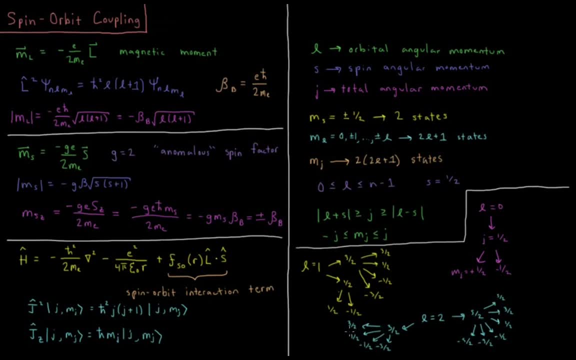 6 values of m sub j, there 4 values of m sub j, there 10 total 2 times 2, plus 1, 2 times 5, 10 total states. So this is the basics of spin-orbit coupling. 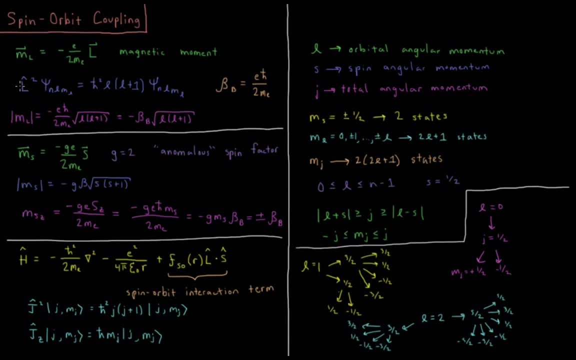 We have our orbital angular momentum operators, Operators and eigenvalues, Our spin angular momentum operators and eigenvalues. Those two combine due to spin-orbit coupling to give us a total angular momentum operators and eigenvalues. We have the value j, going from l plus s to l minus s. 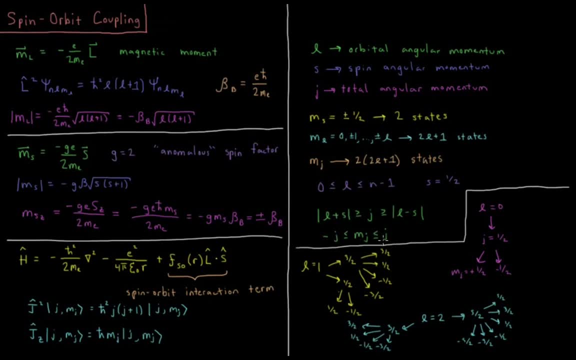 The value m sub j going from minus j up to j. For an electron this is quite simple, because m sub s can only equal plus or minus one half, S is only equal to one half And the values of l are restricted such that we only get two possible values of j for a given. 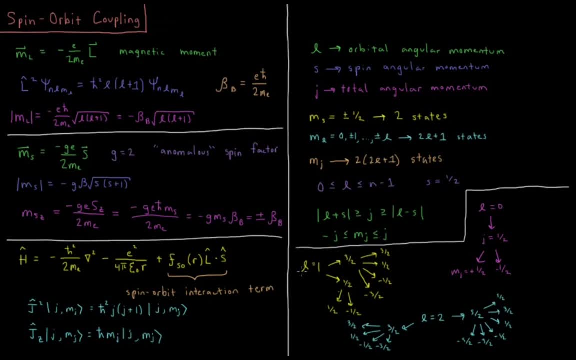 a maximum of two possible values of j for a given electron in a given atomic orbital of a certain orbital angular momentum.